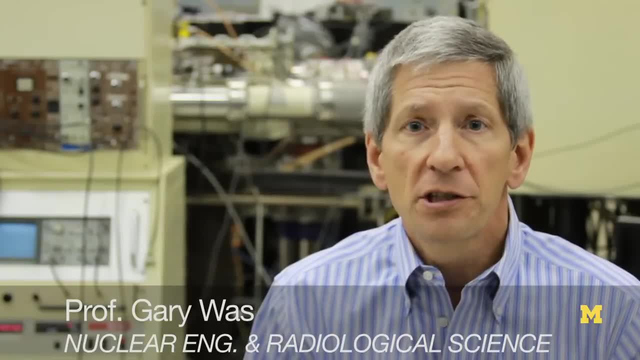 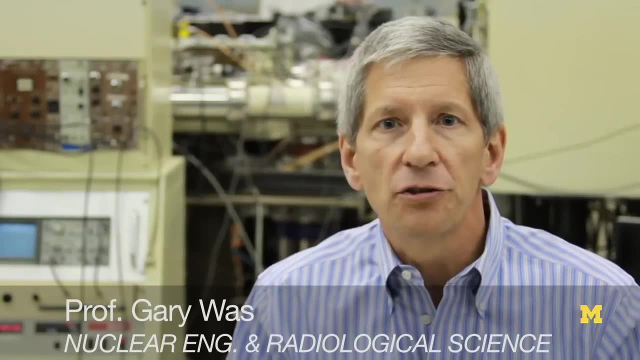 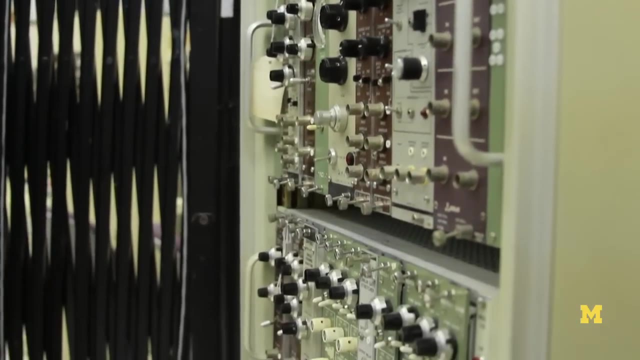 because, first, they're more economical, they're safer, they produce less waste than conventional reactors and they represent the future of an energy source which, again, is carbon-free and very robust in terms of lifetime and economics. The community is also looking at new advanced reactor types: fast reactors. 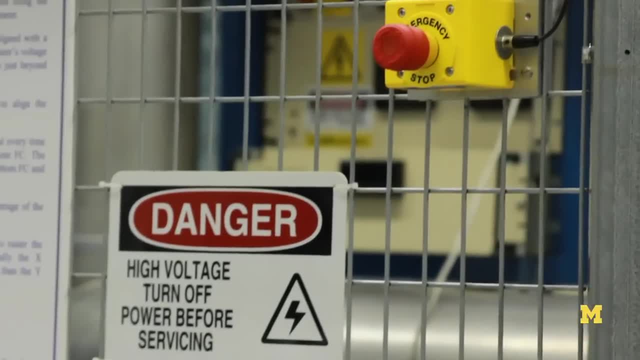 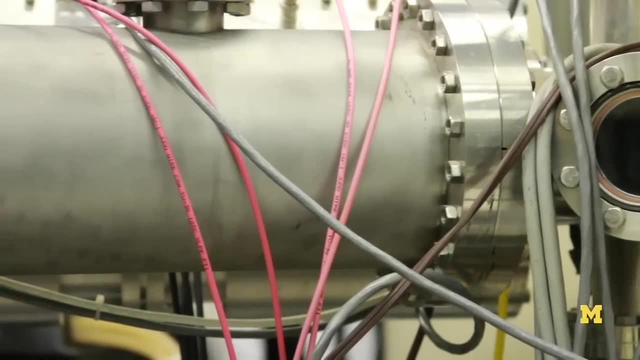 where the radiation damage in cores is even higher levels And those damage levels are very difficult to achieve in test reactors. In fact, in the US we don't have test reactors to get to these levels that we need to get to so that we can understand how materials are going to. 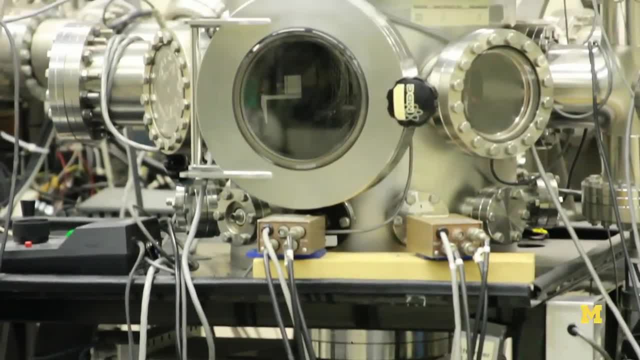 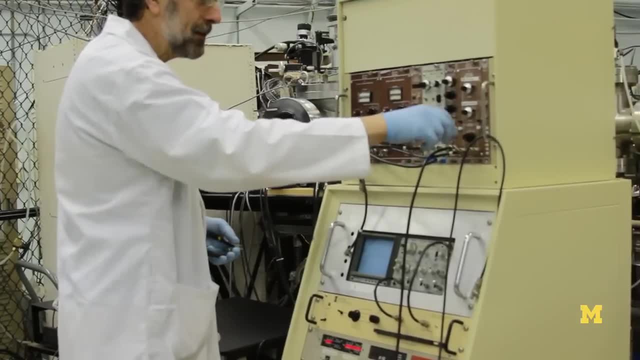 behave. So our approach to this is to use ion accelerators, like the one sitting behind me here. What we do is we simulate radiation effects in a reactor using this accelerator. We simulate the temperature. we simulate the temperature of the reactor. we simulate the temperature of the reactor. 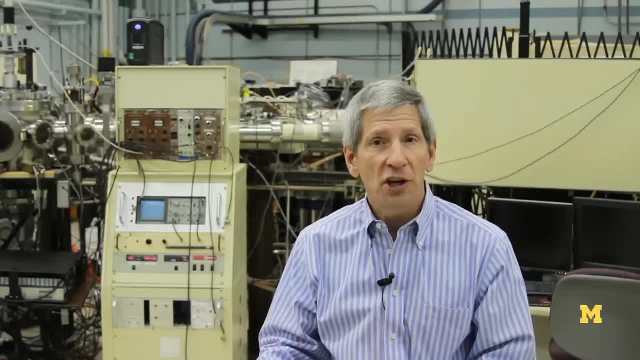 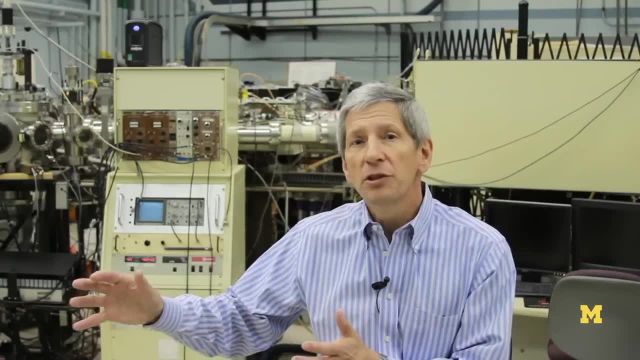 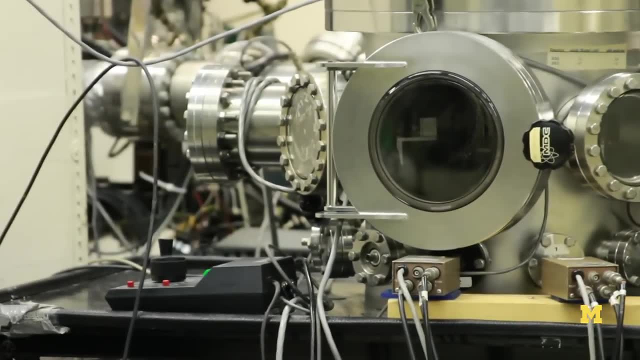 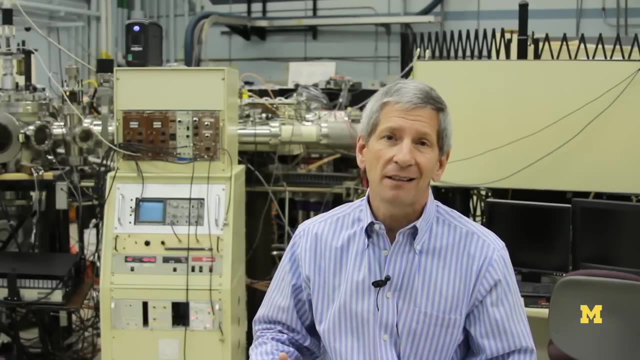 an irradiation such that the resulting structure looks the same after our radiations as it does in a reactor. If we can do that, we'll be able to attack these problems much, much quicker and develop materials and new concepts much quicker. In fact, it'll almost be impossible to do so. 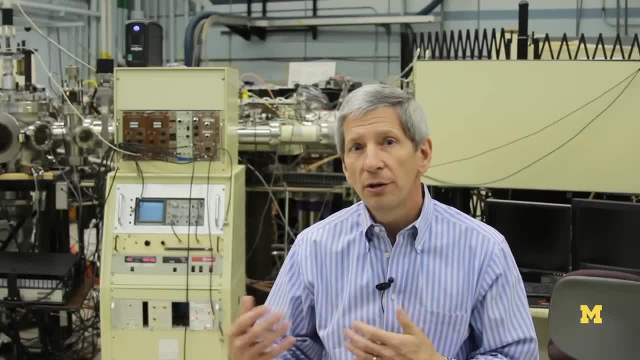 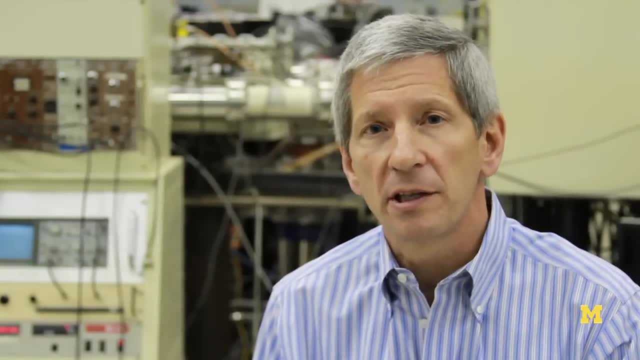 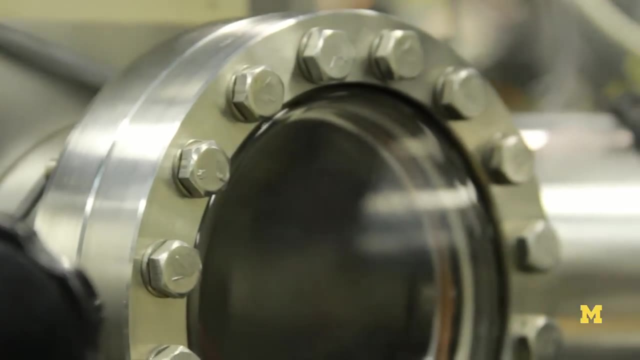 without the ability to use accelerators like this to accelerate the radiation damage phenomena. But we can't simulate everything with one accelerator. It turns out we need multiple accelerators, actually three in total, because under radiation the major things that occur are two: One 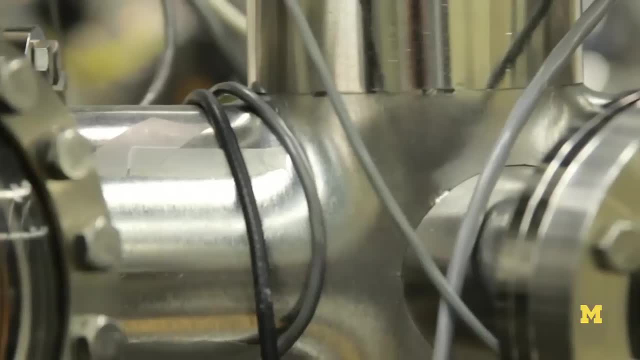 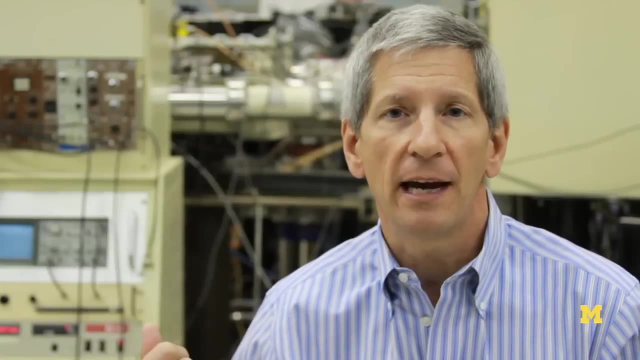 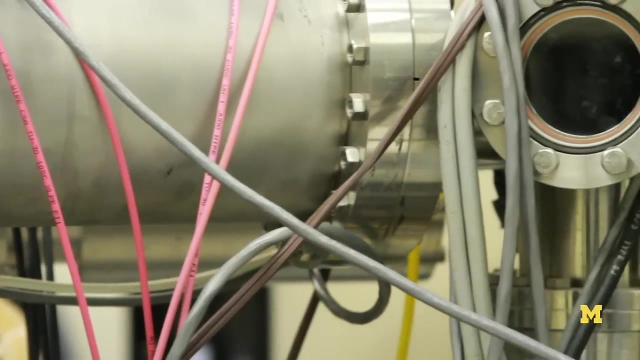 we create damage by displacing atoms and two, we create new materials, new isotopes, by transmutation reactions. So this accelerator can create the damage. We need another accelerator to implant the species that occurs by transmutation in a reactor. So we're redesigning this laboratory. 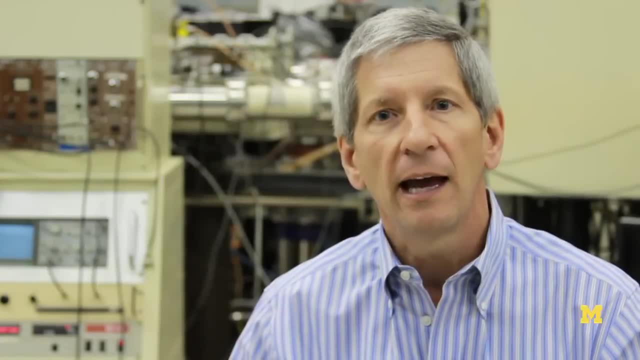 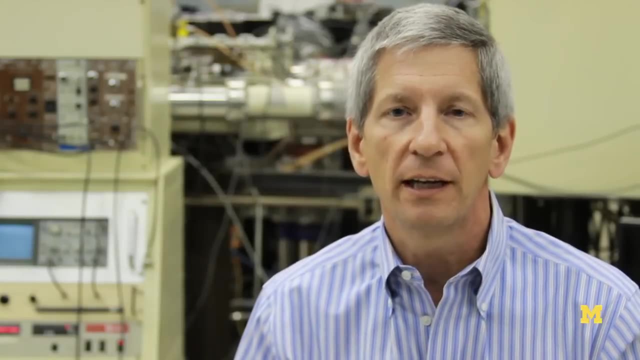 to accommodate three accelerators: the one behind me, the one in front of me and a brand new one that we'll be receiving in November of 2013.. And the objective is to make a national user facility out of this laboratory where we can conduct very high fidelity radiation damage experiments.